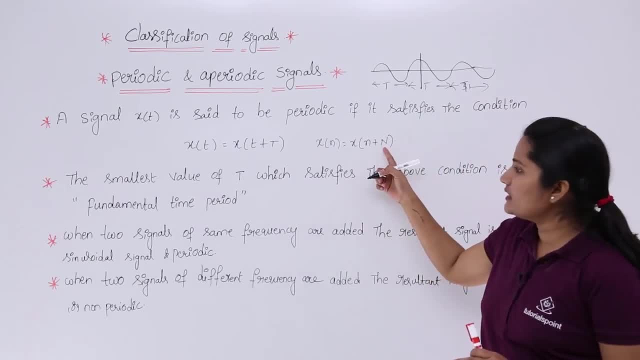 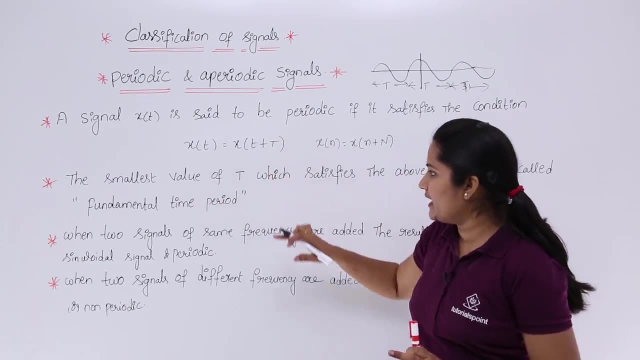 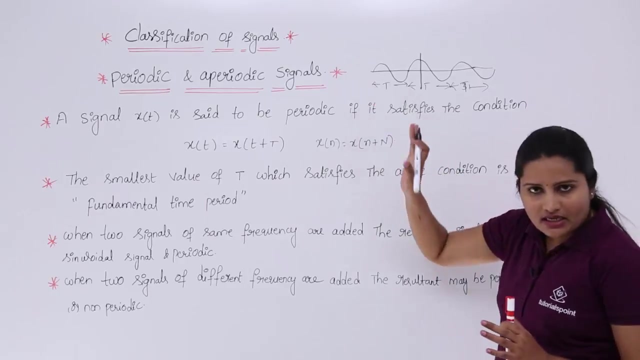 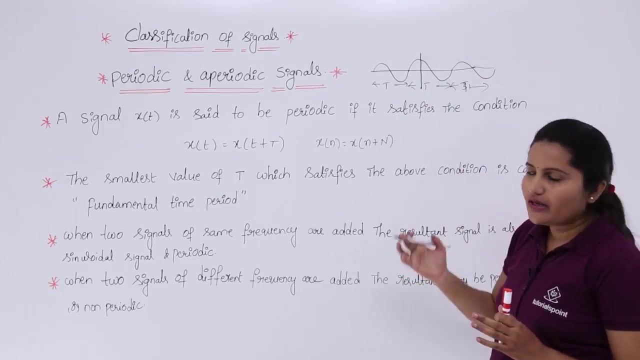 can consider where n is the discrete time period, and here capital N will refers to fundamental time period in discret. So here the smallest value of t which satisfies the above condition is called as fundamental time period. For example, same condition that can be satisfied by 2t, 3t. also, that means x of t equal to x of t plus t, x of t equal to x of t plus 2t. x of t is equivalent to x of t plus 3t. 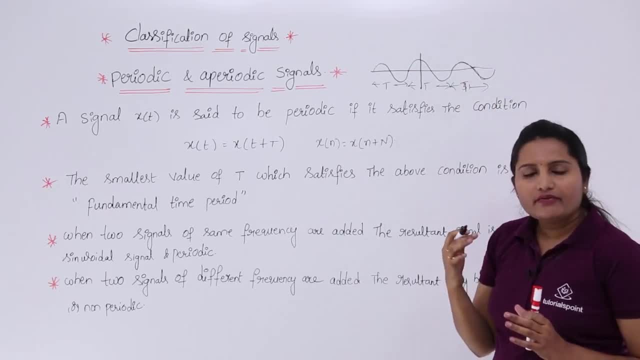 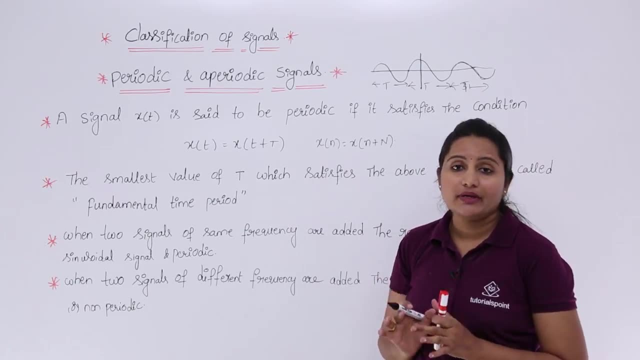 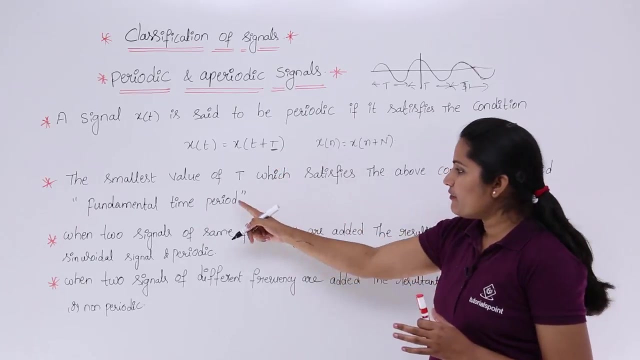 So x of t plus 3t means this signal. So it can be satisfied by different signals, but whatever the least value is there, that is called as fundamental time period. The smallest time period which will satisfy this relation, that is called as fundamental time period. 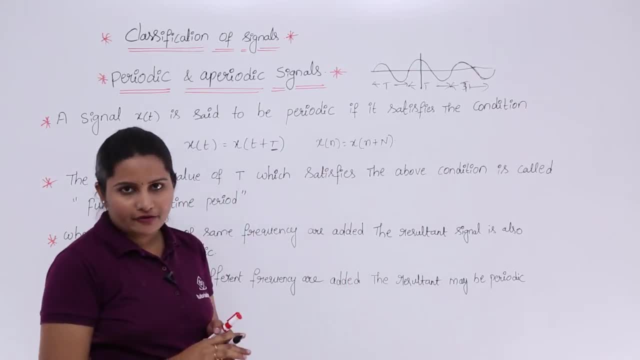 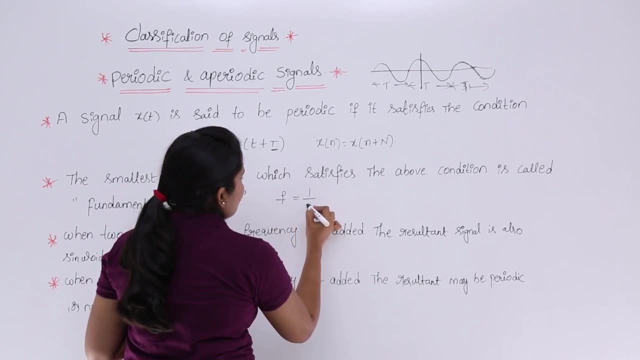 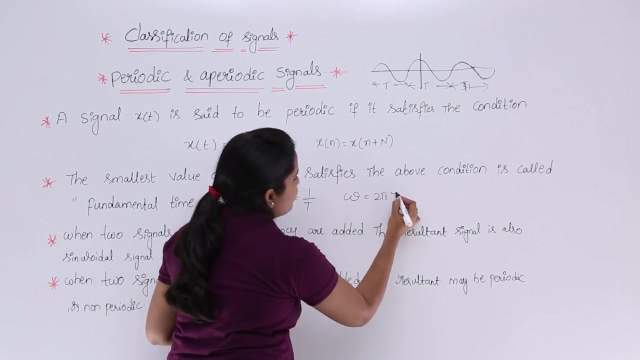 By this time period we can calculate the fundamental frequency also. So here how we will calculate the normal frequency: So 1 by considering 1 by t. You know angular frequency, omega is equivalent to 2 pi f. So 2 pi f means if you substituted this 1 by t here, then you will get 2 pi by t. 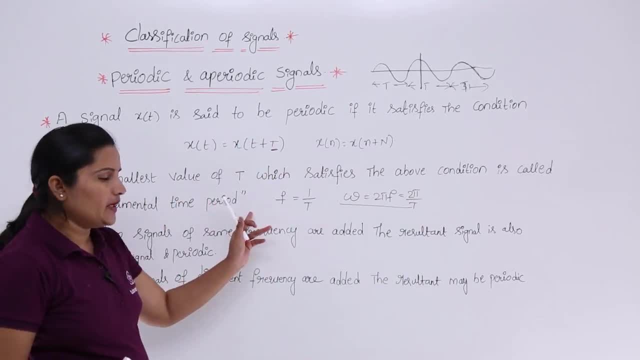 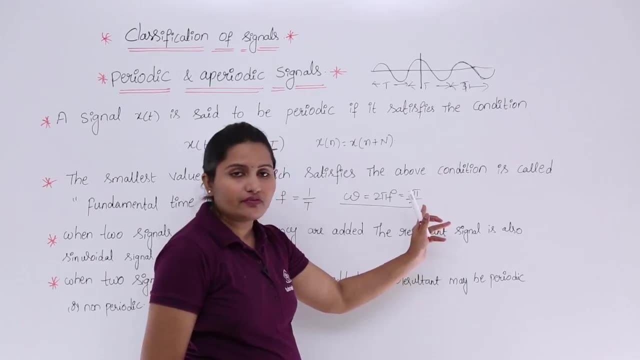 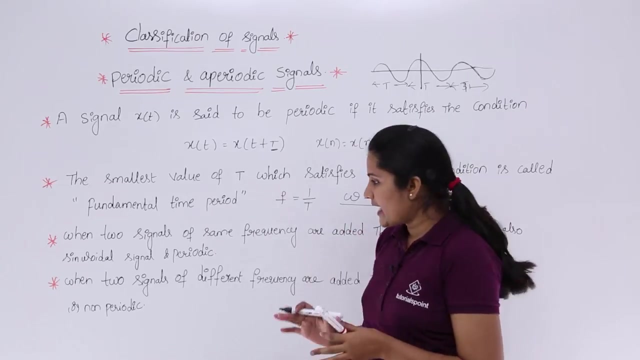 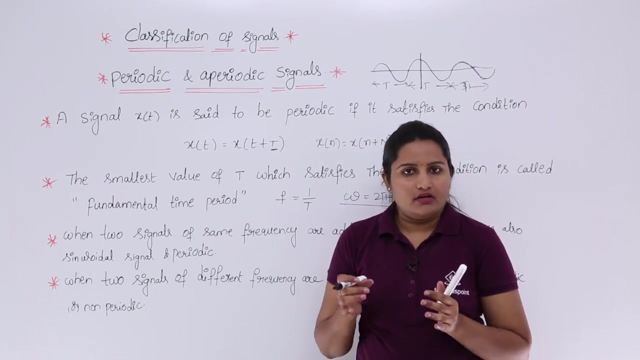 So now, by having knowledge about fundamental time period, you can calculate your frequency of the signal and your angular or fundamental frequency of the signal 2 pi by t, like this. So now we are having some important points about this periodicity. When two signals, when two periodic sinusoids are added, the result is actually a sinusoidal signal, definitely a sinusoidal signal and is periodic also. 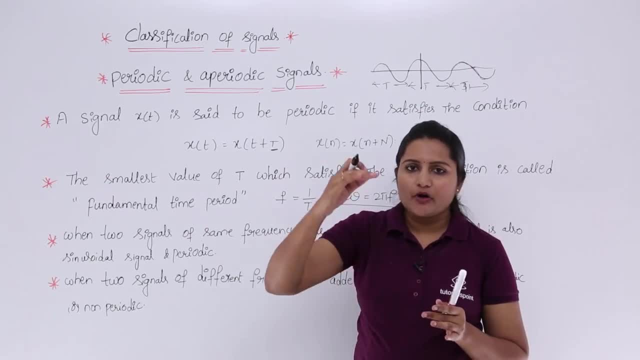 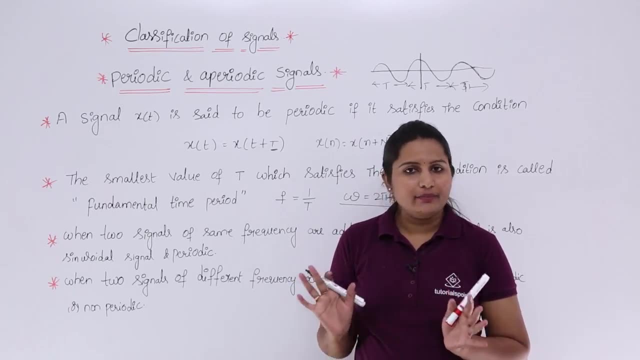 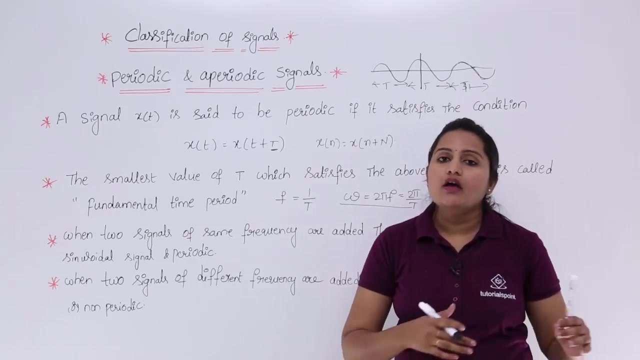 When two signals of same frequency added, so corresponding amplitudes are going to add and result is definitely a sinusoidal signal and is said to be periodic. When two signals of different frequency are added, different frequency signals, for example, one signal is having 2 megahertz, another signal is having some 4 megahertz.